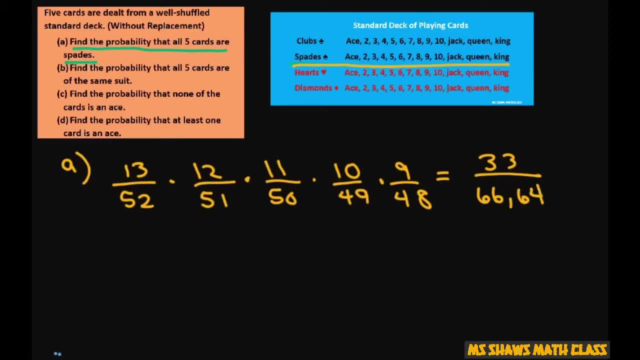 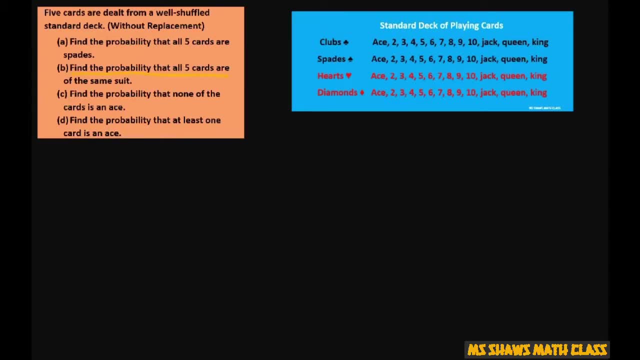 by 66,640.. Okay, Next one: Find the probability that all five cards are the same suit. So for this one, what we want to do is find the probability that Let's just say, for our first one, five spades. for the first one, we did A, we got. 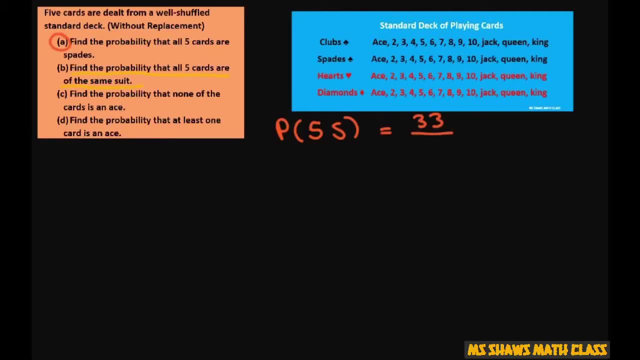 63,640.. So basically that's going to happen on all these suits. So for our probability of five of any suits, that's going to be basically a probability of five hearts plus probability of five diamonds plus probability of five. 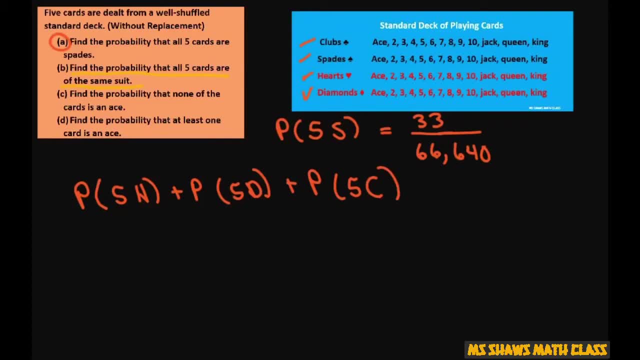 clubs, plus probability of five spades. So we're just going to use this. We already know that they're all going to be the same, So that's just going to be. since we have one, two, three, four suits, that's going. 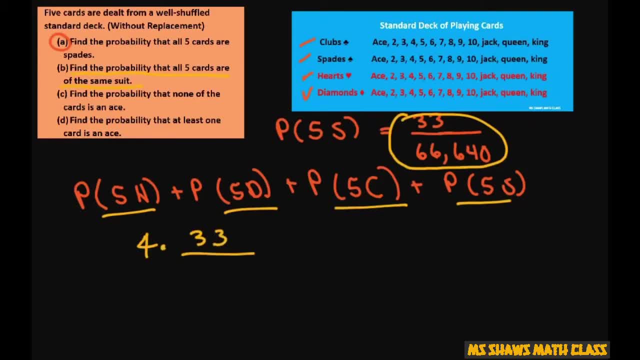 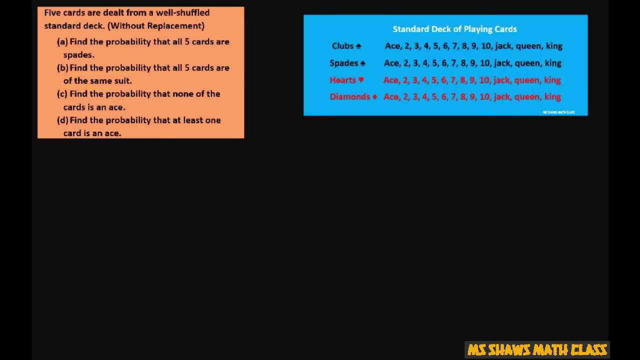 to be four times 33, divided by 66,640.. And that reduces to 33,016,660.. All right, And then number C or letter C. find the probability that none of the cards is an ace, So no ace. 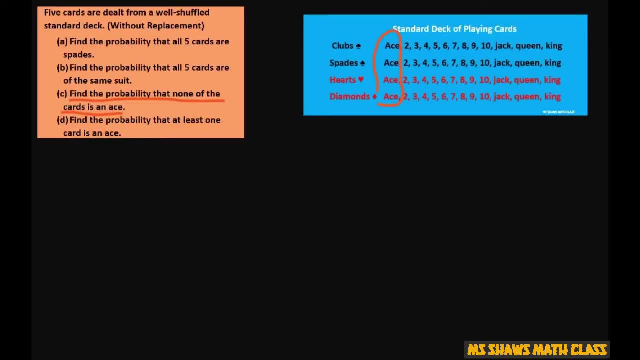 If there are no aces, we have a total of four aces here. So 52 minus 4 is 48. So we're going to do: probability of no ace equals 48 divided by 52 times 47, divided by times 46, divided by 50, times 45, divided by 49, times 44, divided by 48, which equals.